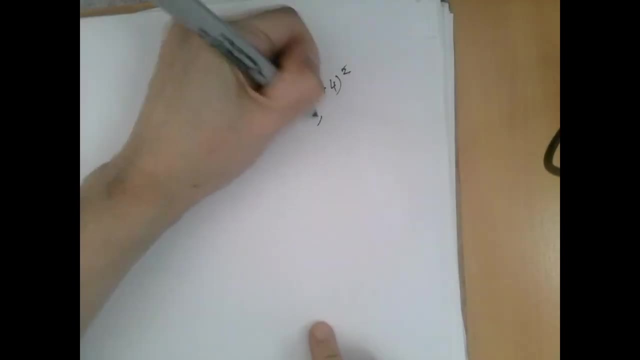 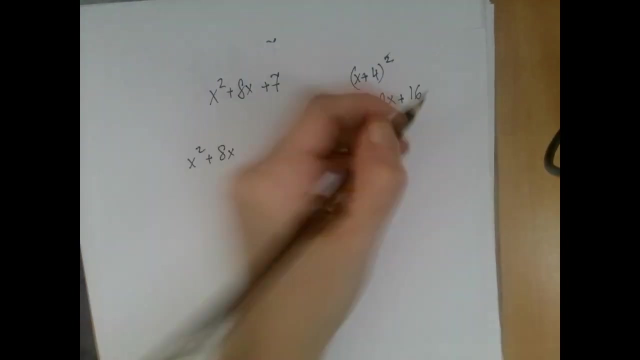 x plus 4 squared And when we expand it we get x squared plus 4x. plus 4x gives us 8x plus 16.. So we're going to smuggle in the 16 to have the complete square. So the first three terms gets: 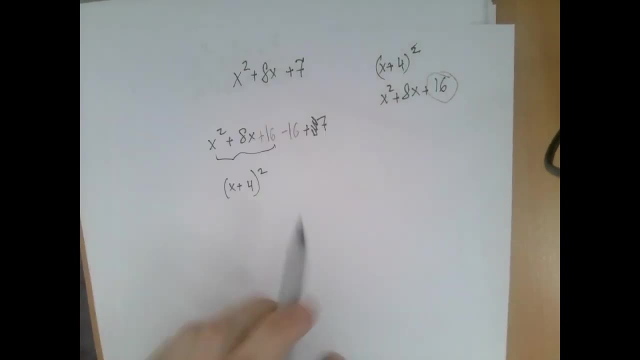 absorbed x plus 4 squared And negative 16 and plus 7 combines into negative 9, which is good news. It's a square. So we have x plus 4 plus 3 times x plus 4 minus 3.. 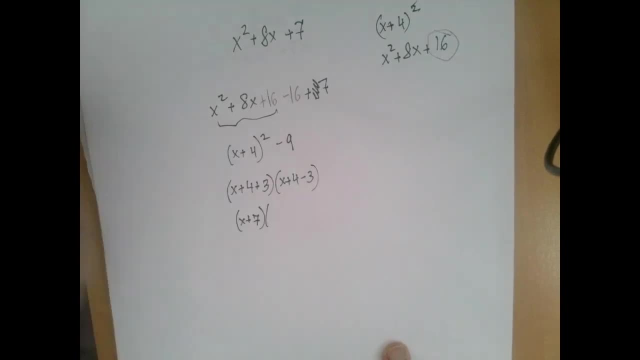 Which cleans up as x plus 7 times x plus 1.. No one is really surprised. We sort of knew where this was going. Okay, so we can rewrite now the numerator as x plus 7 times x plus 1.. The only 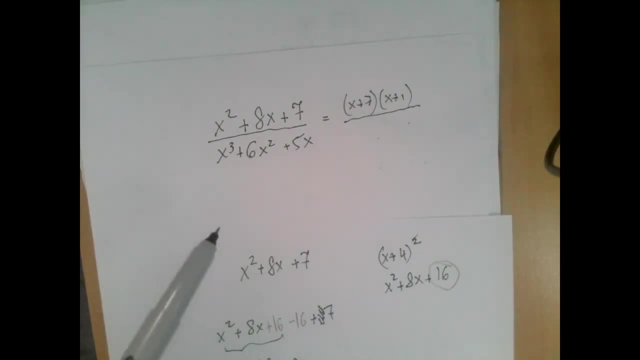 way we can simplify this rational expression, if first the denominator can be factored and one of the factors is one of these. Otherwise we cannot simplify it. Let's see this one. So notice it's cubic, but it's not really because x can come out. So it's not really because x can come out. So if you 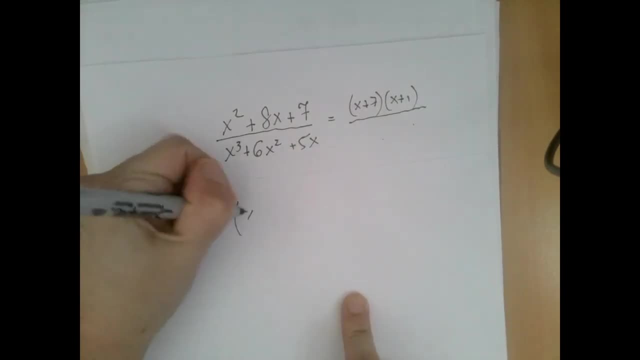 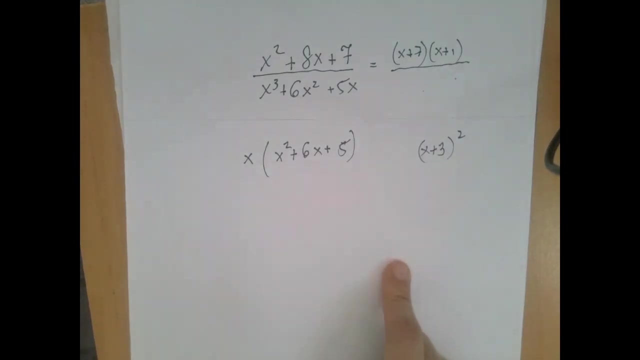 factor out the greatest common factor, x, we get x times x squared plus 6x plus 5, which is also a fairly easy thing to factor. So half of the linear coefficient is plus 3.. So we're going to expand x plus 3 squared, which is going to be x squared plus 6x plus 9.. So we're 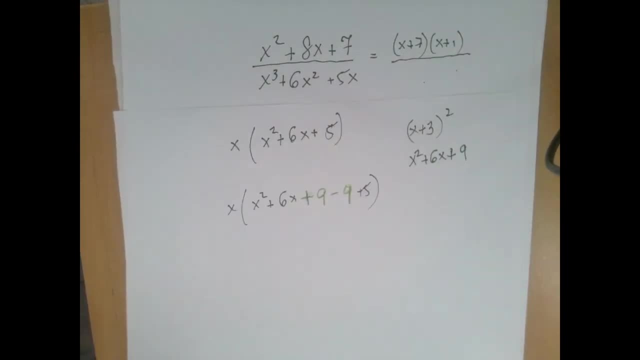 going to smuggle in the plus 9.. And so the first 3 gets absorbed into the complete square, x plus 3 squared. And then we combine negative 9 and plus 5. And that's negative 4, which is good news. 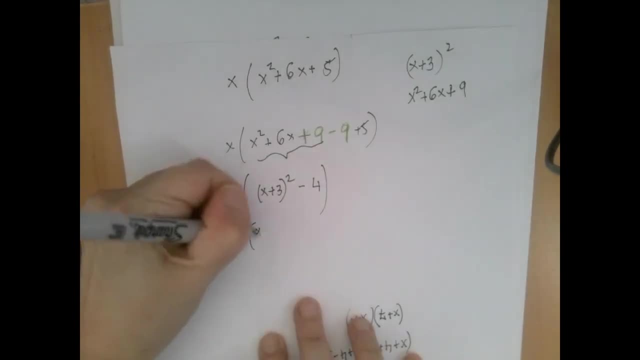 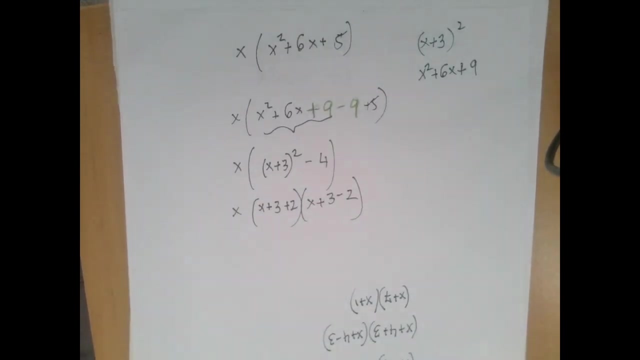 because it's a square. So we have x times x plus 3 plus 2, x plus 3 minus 2.. Notice that we skipped a few steps. So we can speed up as we become experts in completing the square. So what we? 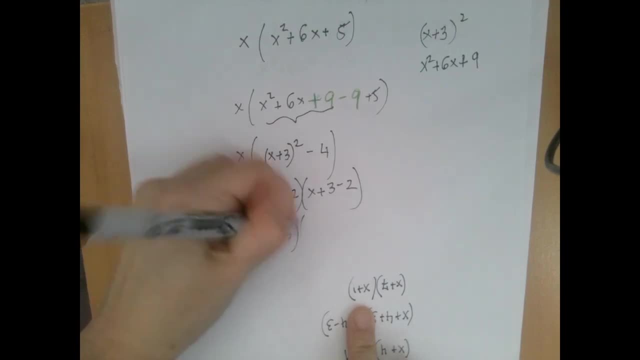 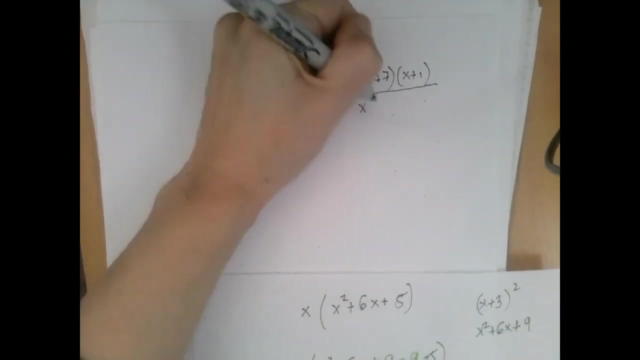 have is x times x plus 5 times x plus 1.. So we go back to our fraction rational expression, And the denominator is x times x plus 5 times x plus 1.. And so the only thing that will cancel out is x.